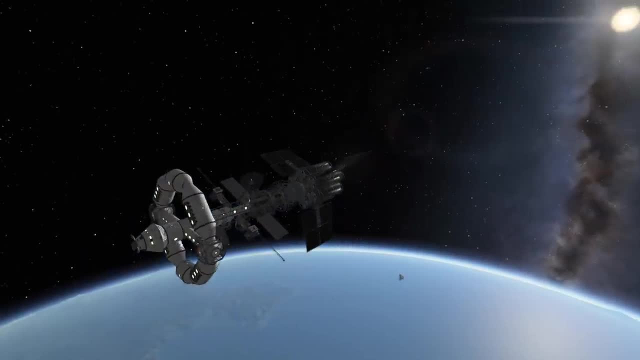 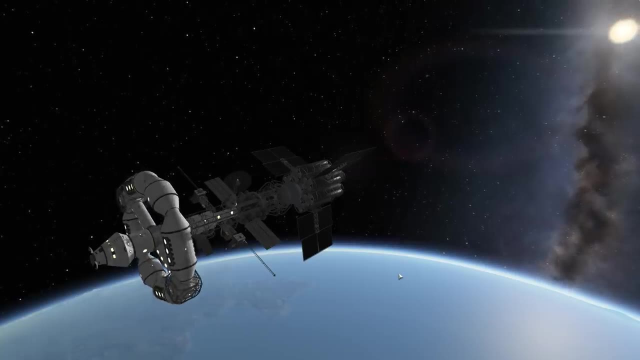 factor how much extra energy you get out from the fusion compared to the energy that you put into making the fusion start. So they calculate they need a gain factor of about 200.. And to get the gain factor of about 200, they would need for a seven-month Mars mission. they would need something. 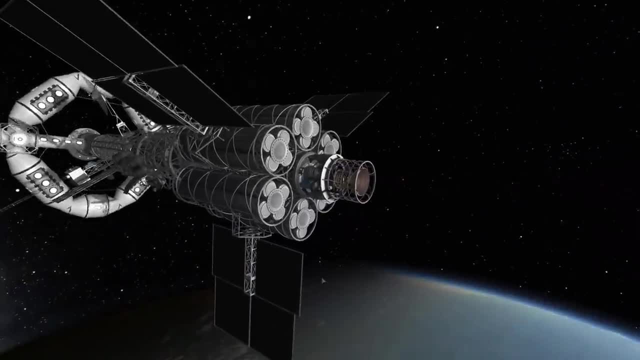 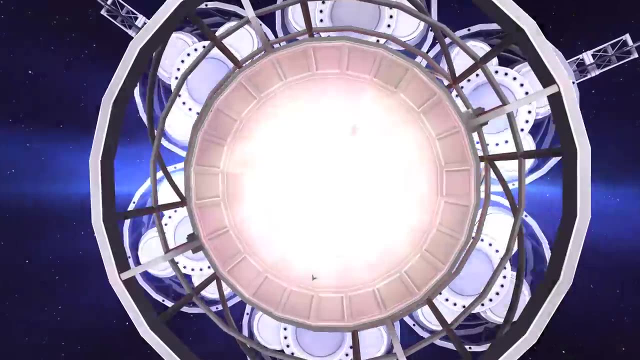 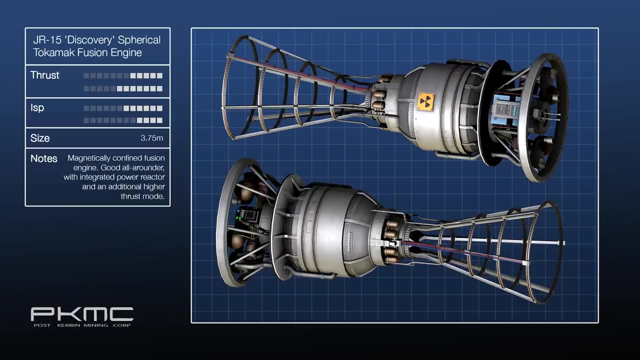 like 400 kilowatts of solar panels to power this drive system. So I mean it would obviously be revolutionary. In fact, any of the drives covered in this little episode would be revolutionary. So let's go to the next one, The Discovery Spherical Tokamak Fusion Engine. So this is. 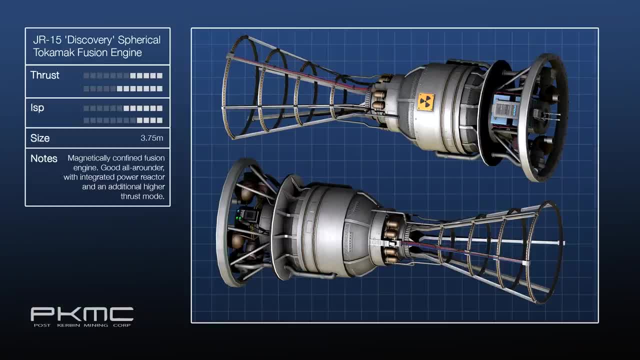 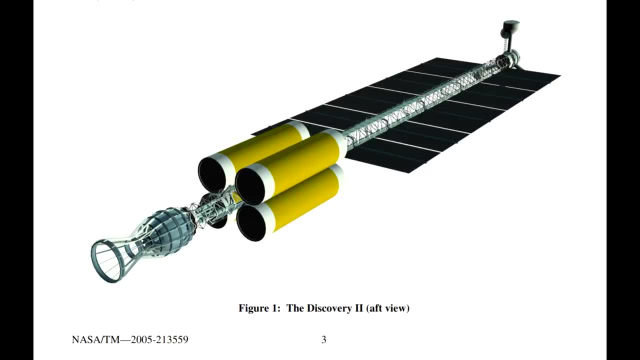 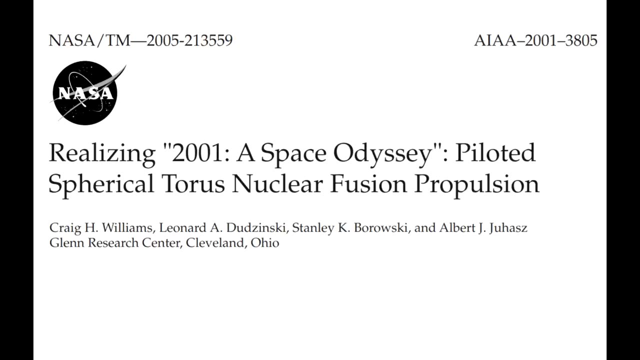 actually based on a hypothetical engine from a NASA study looking at a crewed mission to Saturn, right? So this is their Discovery 2 with a habitation module with rotation at the far end, And, yeah, I think this is from 2001.. They're actually literally trying to do 2001.. Now the 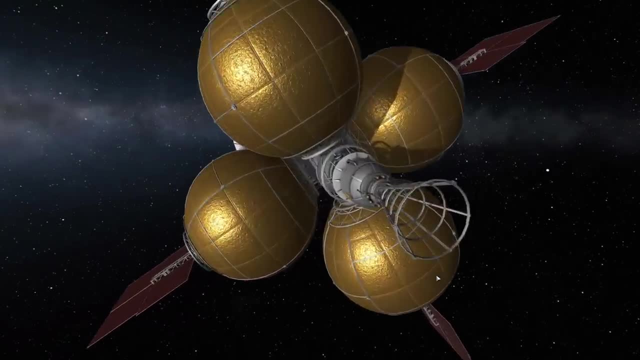 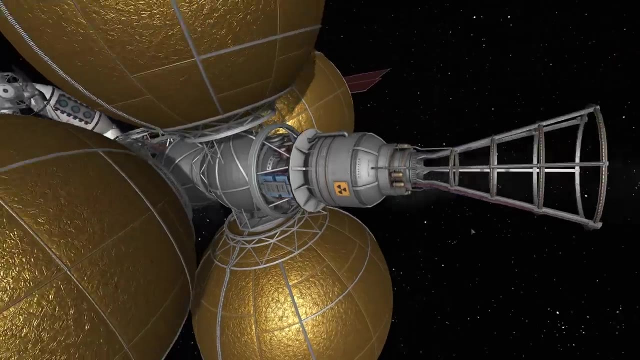 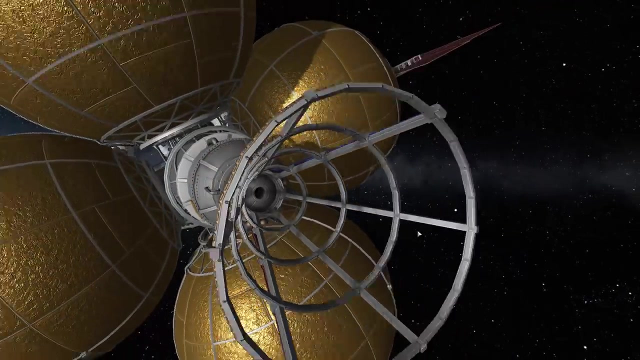 Spherical Tokamak Park tells us that this is a magnetic confinement fusion system, which is where you try to compress and confine the plasma using magnetic fields. It sounds easy enough: you sculpt a piece of jelly into a useful shape using only rubber bands. When you start to try to 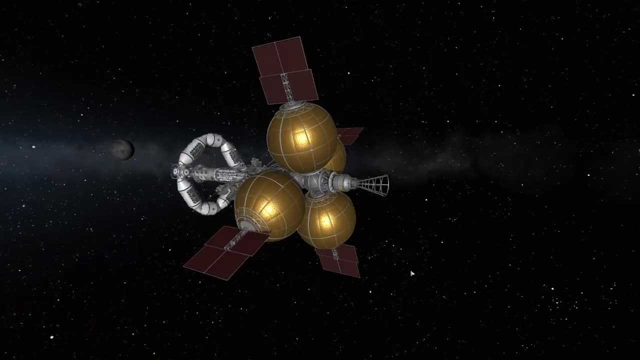 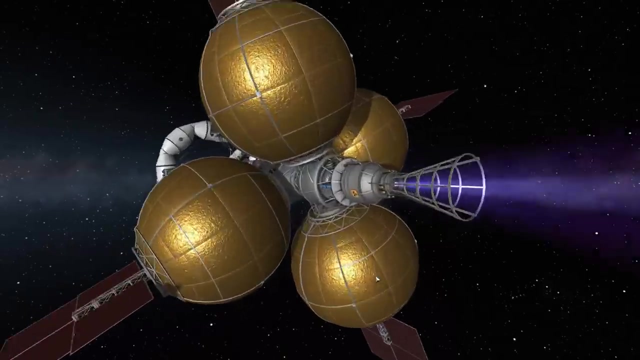 apply real pressure, the contents have a habit of leaking out and messing up your lines of force. But one of the research, one of the sort of core things you find in plasma research, is the tokamak, which is something which holds a plasma in a magnetic field. that is shaped like a donut. 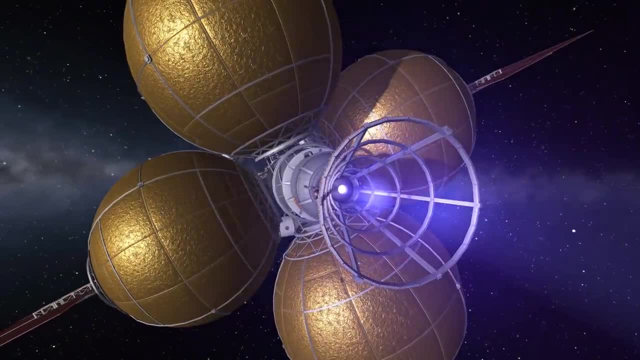 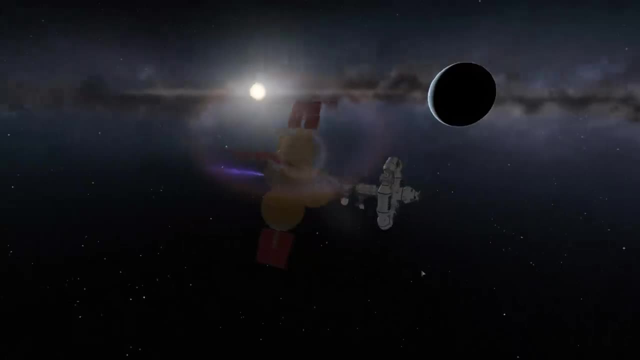 So a spherical tokamak is where you kind of take the donut, you squish it, so the hole in the middle of the donut is as thin as possible, like a big vertical cylinder, and you squeeze it into a spherical shape. So the idea I guess with these engines 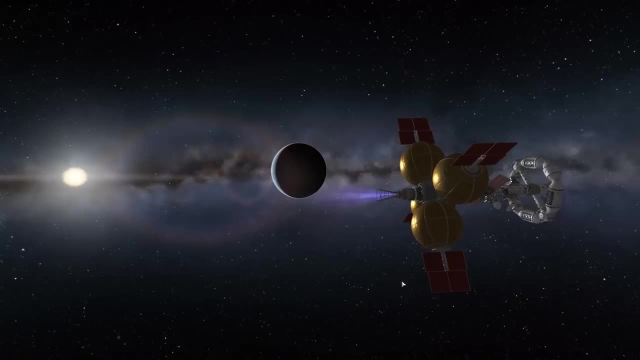 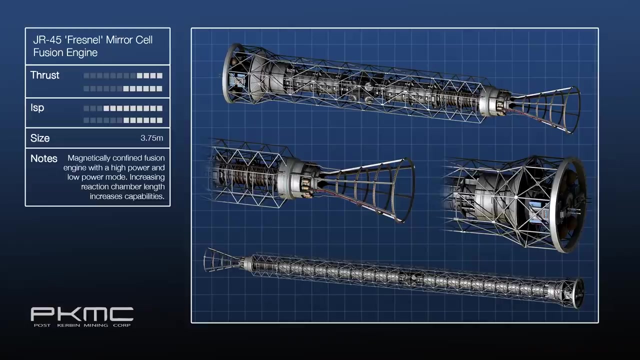 is that you have a reaction chamber where you've got a confined plasma, you've got fusion happening and then you allow it to leak out as a rocket exhaust. So your energy is coming from the fusion and your exhaust is coming from the plasma that is being heated up and leaking out. So the mirror. 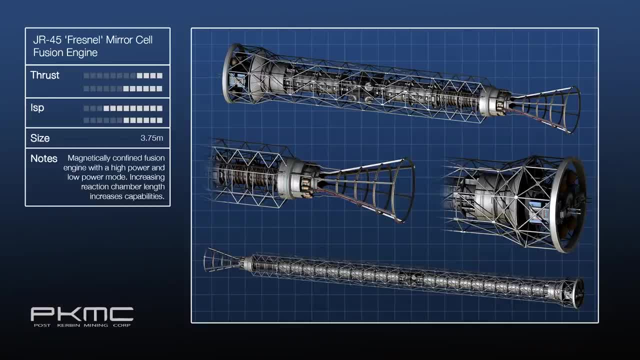 cell fusion engine is a rocket engine. It's a rocket engine. It's a rocket engine. It's a rocket engine. It uses the same magnetic confinement system, but instead of it being in a donut shape, they just have it in a long, thin chamber. In the mod, you can actually have the chambers be very. 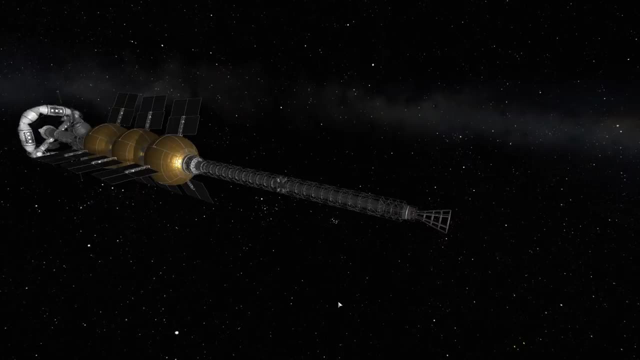 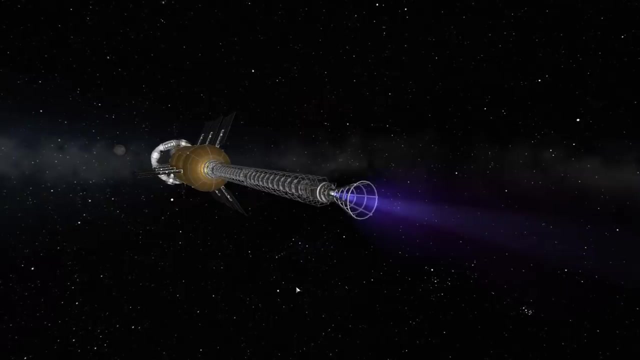 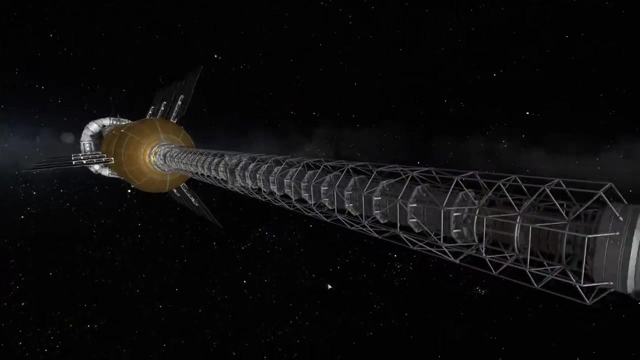 long, like 45 meters long, and you have a magnetic mirror at each end to kind of confine the plasma and stop it leaking out the ends, except that you make the geometry subtly different on one end so that it can leak out and provide you thrust. Now, in this case we actually have another advantage. 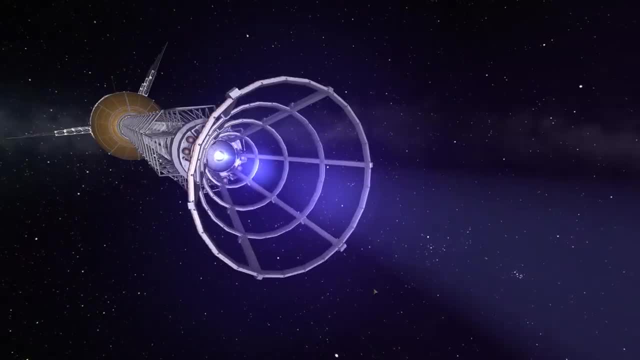 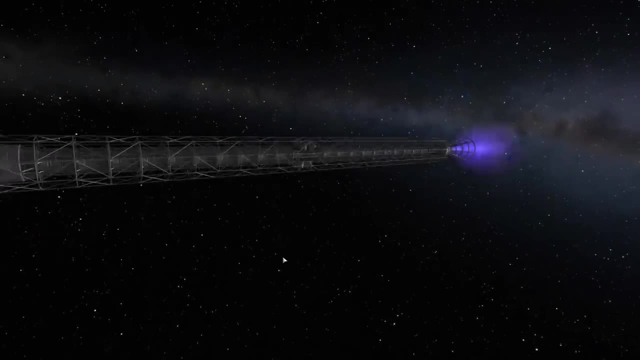 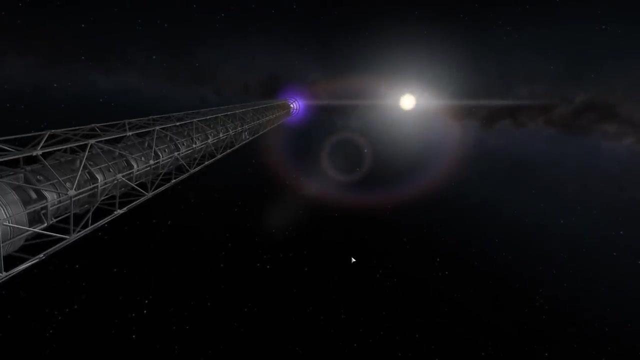 where you can use the heat and that plasma to heat regular liquid hydrogen, the boring old hydrogen that doesn't really undergo fusion unless it's in the middle of a star. So by doing this you're dumping extra mass into the exhaust and it's getting heated up, So you get much higher. 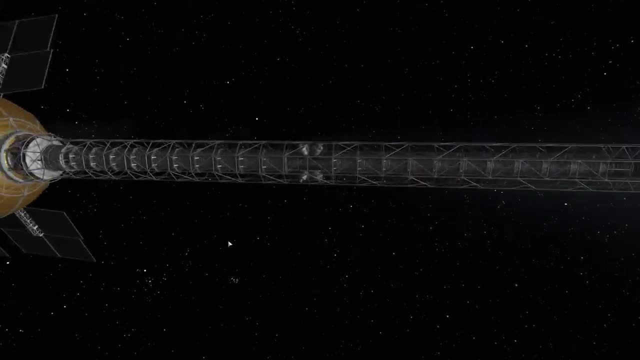 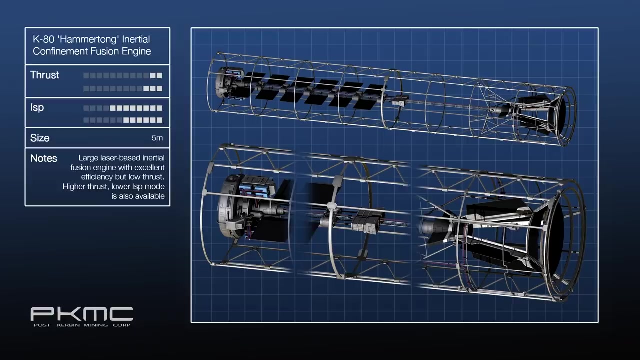 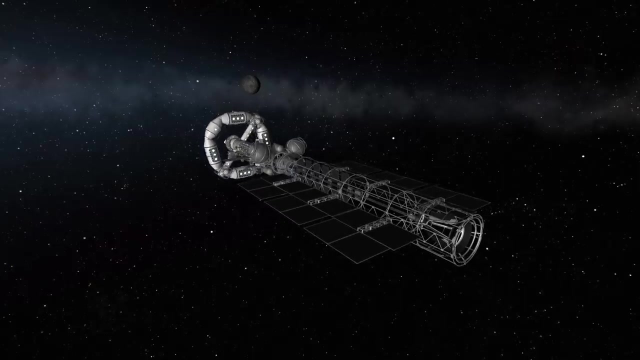 thrusts at the expense of lower specific impulse. Now we have the hammer-tongue inertial confinement fusion engine. So inertial confinement doesn't use magnetic fields. What it does is it tries to squeeze it and it squeezes it using a bunch of lasers. So this drive. 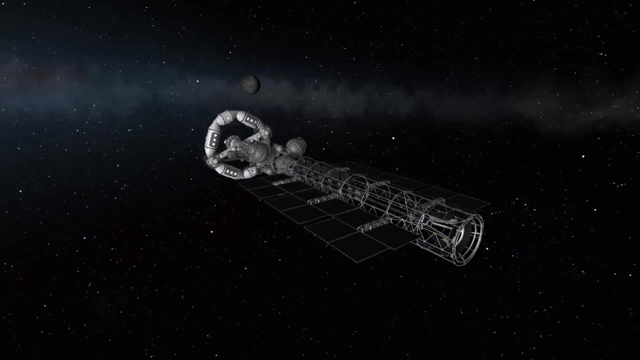 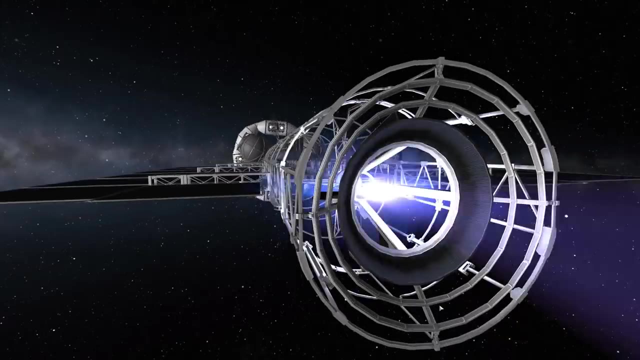 in terms of game technology. it produces these little fusion pulses which are triggered by a lot of lasers being fired at a tiny pellet, And you can actually see the lasers in the model focusing on the pellet, causing it to explode. Now, to actually make fusion happen, you have 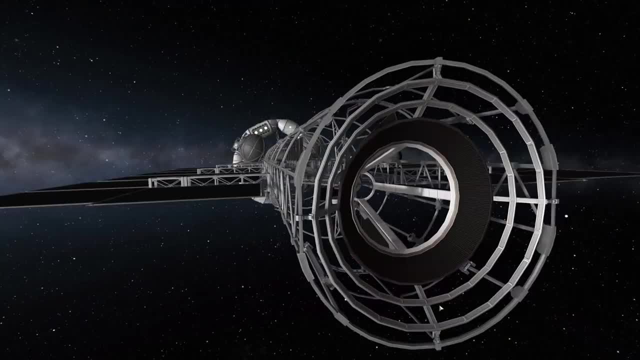 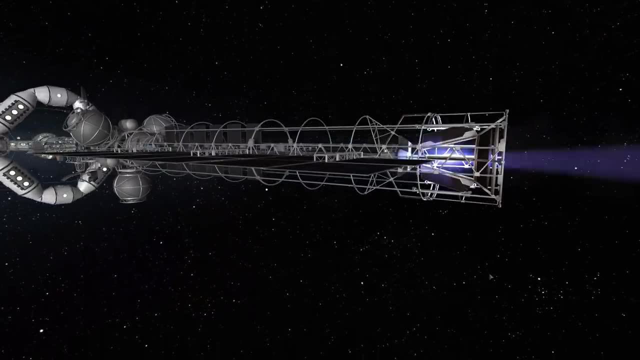 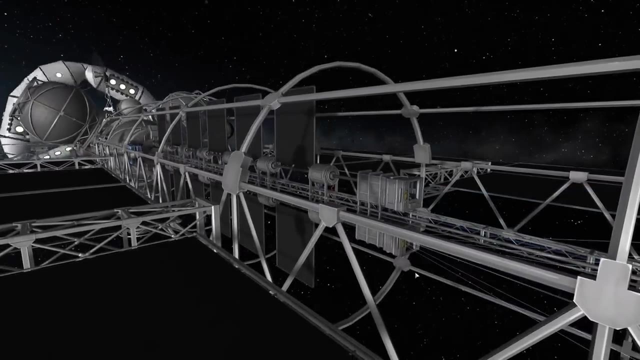 to compress it and heat it up. And you can see that with lasers it's very easy to heat things up. But how do they compress it? Well, the surface layers of that pellet boil off and evaporate And it's like the impulse from a rocket blowing off and squeezing the pellet down, causing the 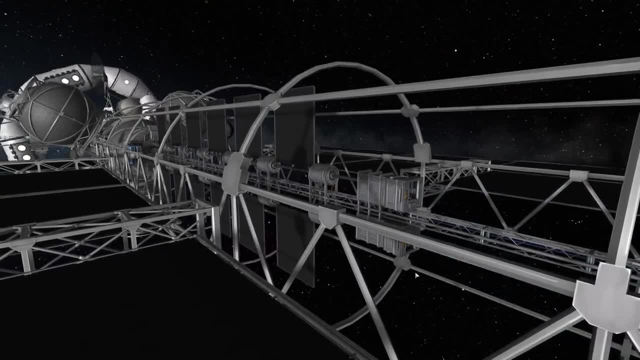 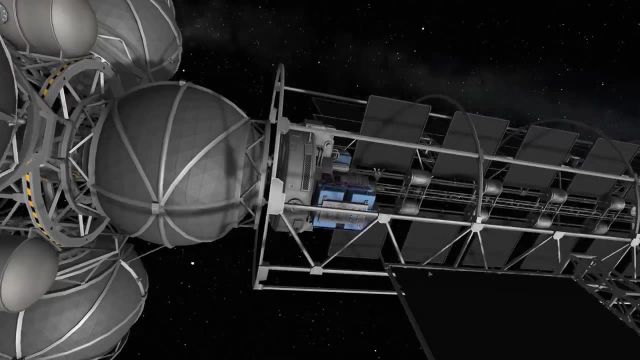 explosion. This is something that is actually done for real. There's the National Ignition Facility, which is close to me in California, where they have a giant building where they do this exact thing. I mean, they don't fly the building around, They just have a giant building. 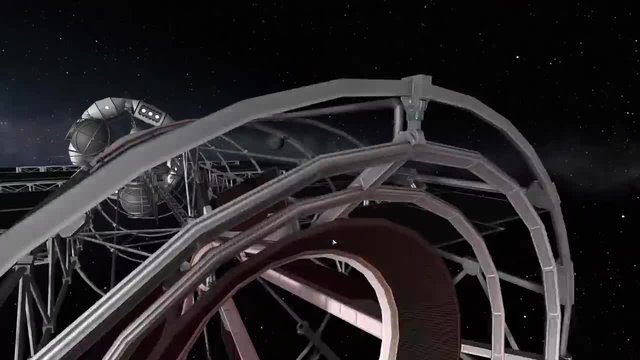 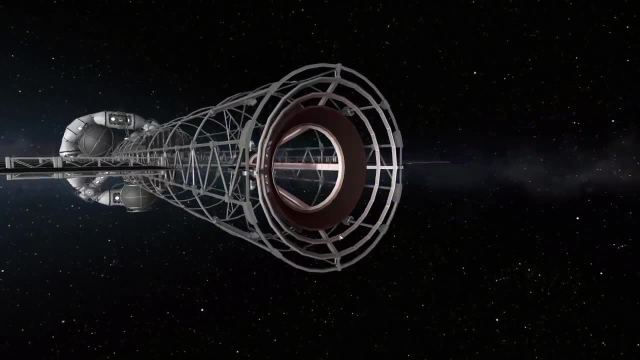 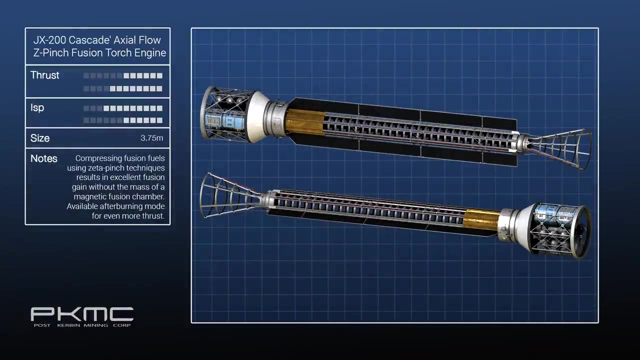 where they cause tiny pellets of nuclear material to explode. And the reason they do this is so they can study the behavior of thermonuclear weapons without actually detonating a real thermonuclear weapon. That's why the test band treaty is actually a very good thing for the US. So now we have the Axial Flow Z-Pinch Fusion Torch Engine, The Z. 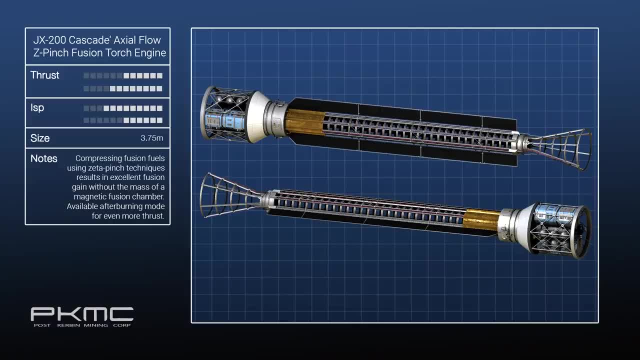 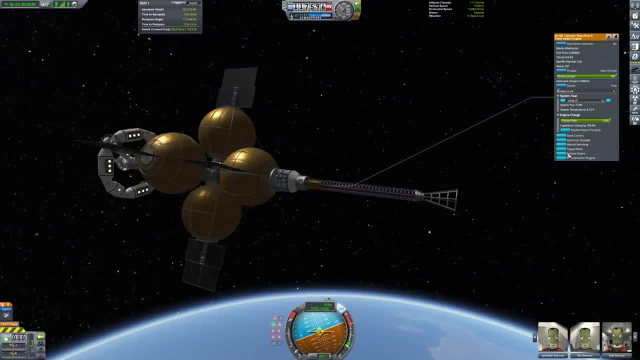 is for Zeta. It basically implies a mechanism where you flow electricity through the plasma because it's conducting, And that generates a magnetic field that spirals around the outside And that can be used to generate a magnetic field that spirals around the outside. 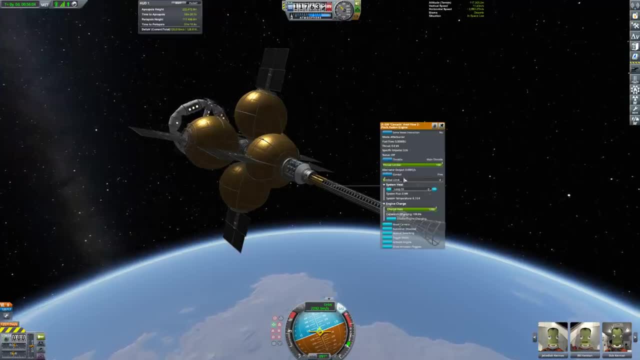 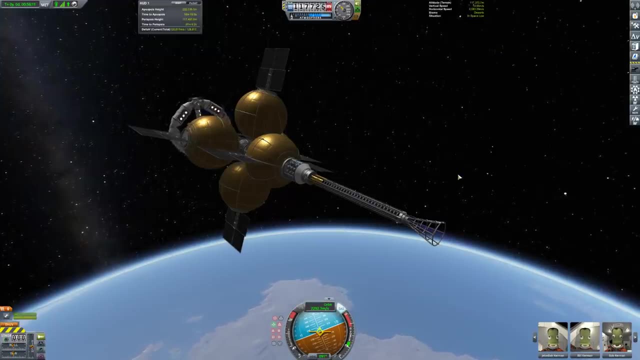 And that can actually be used to compress the contents of the plasma. This was one of the ideas for very early fusion systems. However, this is inherently unstable And you would inevitably end up with things flying around and falling apart, But there are ideas where you can create. 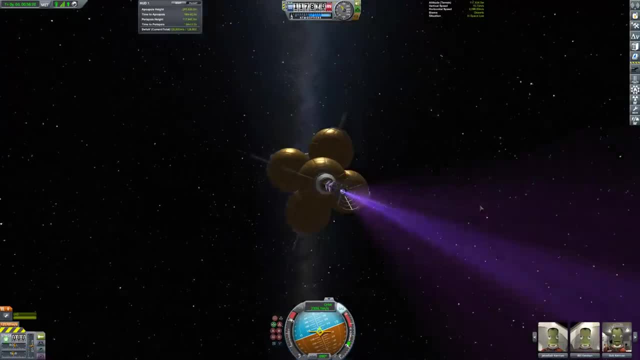 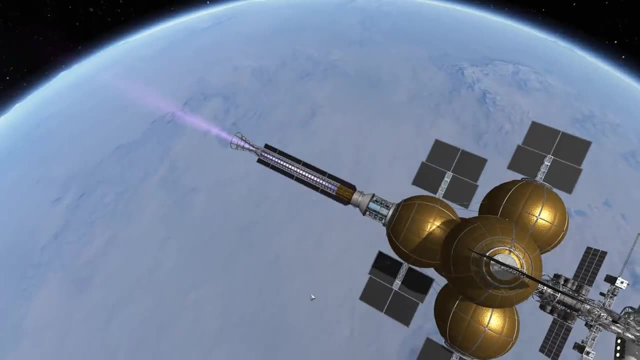 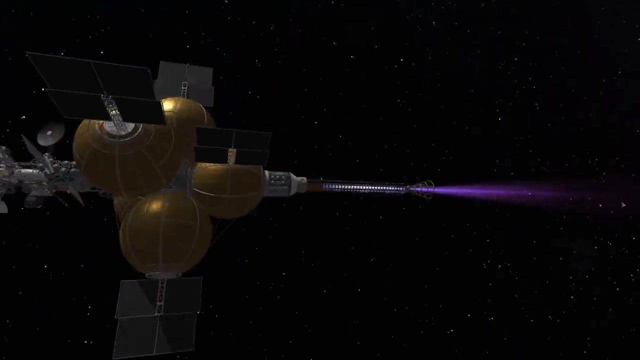 a very, very long, thin plasma, run the current down it and cause the plasma to collapse and generate your fusion power. Now, this one is only tens of meters long, But the ship's that I've seen from studies that use this, like the Firefly by Icarus Interstellar, that's like 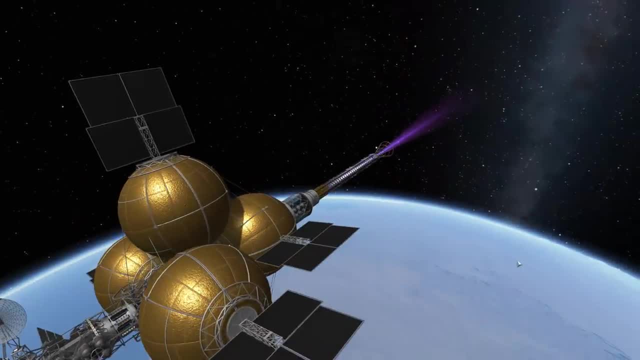 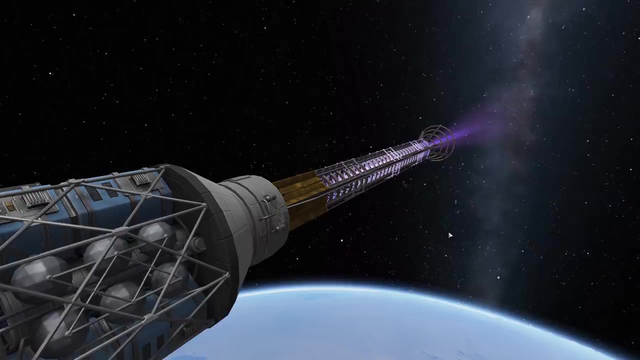 a kilometer long In the mod. this is supposed to be the best one available to you. So it also adds an afterburning mode where you can dump extra hydrogen in it to get high thrust. Or you can just use the pure deuterium and get really good specific impulse, But actually before you get 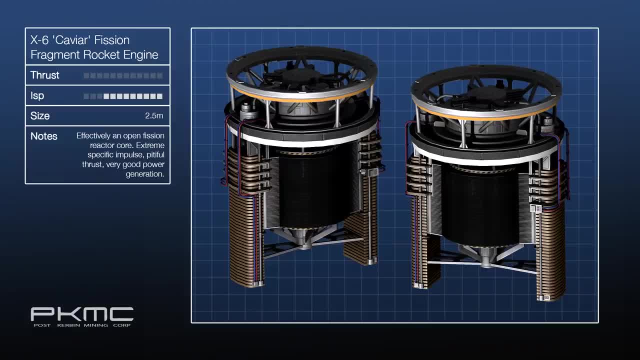 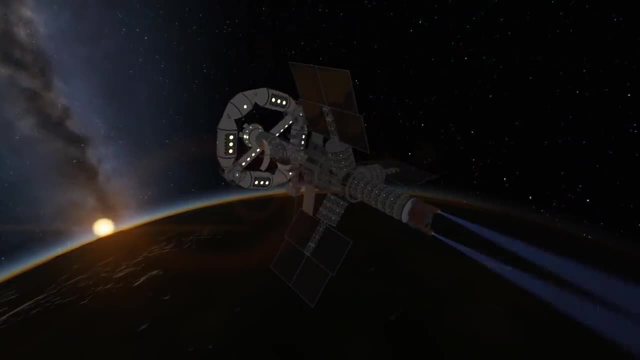 the fusion tech, you get fission, And this is the Caviar Fission Fragment Rocket- Again, real concept. The idea behind a fission fragment rocket is that you're using a nuclear reactor to a fission reactor And, as you have fission events happening, the daughter products that get knocked out of the 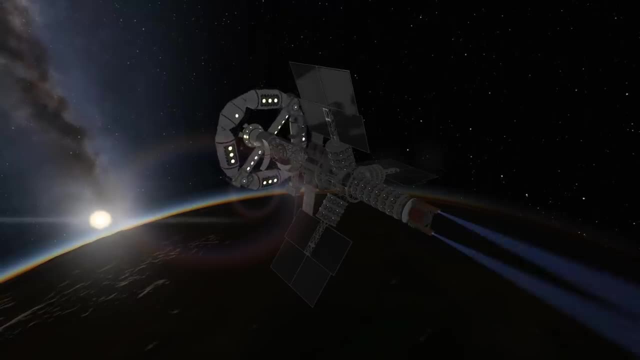 uranium. those are ionized And they are very high energy. So you capture these particles using magnetic fields and electric fields And that is your rocket exhaust. Now it's kind of hard to build a reactor that works like this, because critical masses tend to prefer all your. 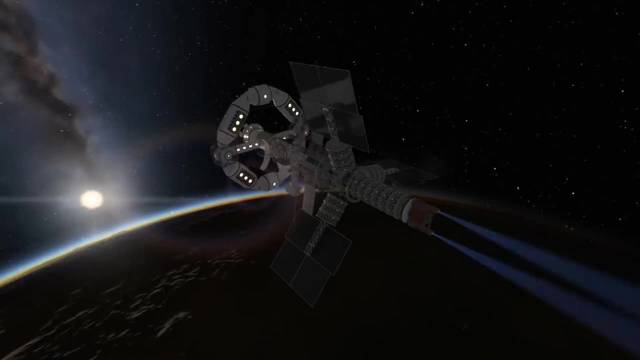 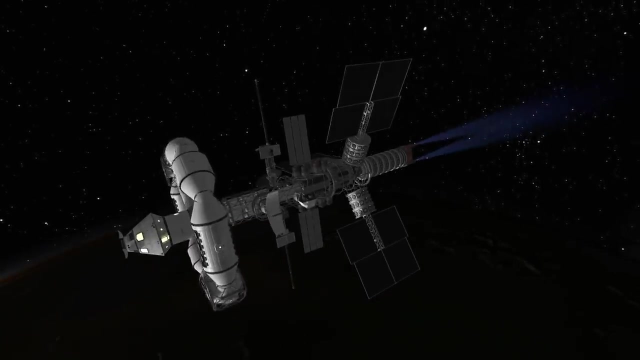 material to be in one solid lump, Because a critical mass for a fission depends upon the geometry of the mass that you have. But if you want to harness the fission products for rocket exhaust, then you want the fissions to be happening near the surface. So you need a structure that has 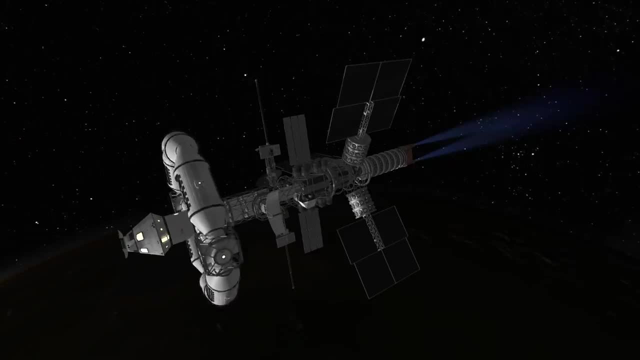 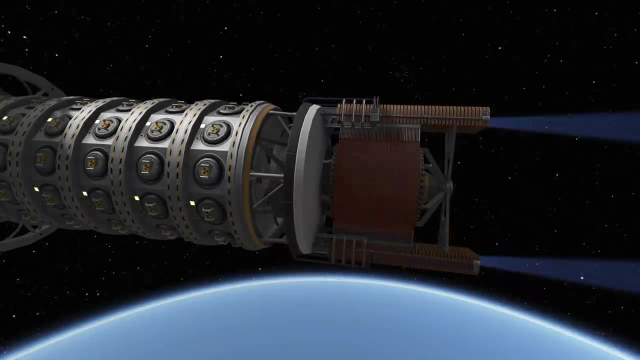 a very high surface area and also a sufficient critical mass, And, furthermore, the surfaces can't have to be exposed to the vacuum. They can't have cooling fluids running over it. So this is one of the things that we're going to be looking at in the future, And this is one of the 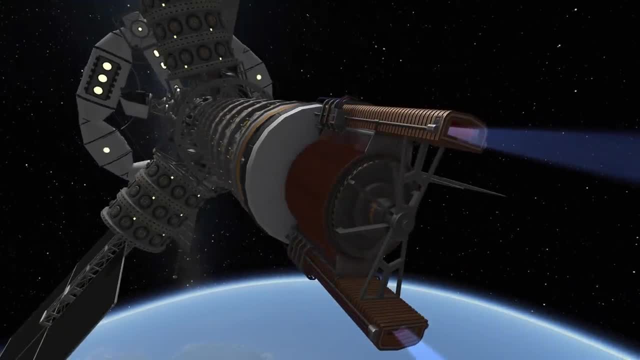 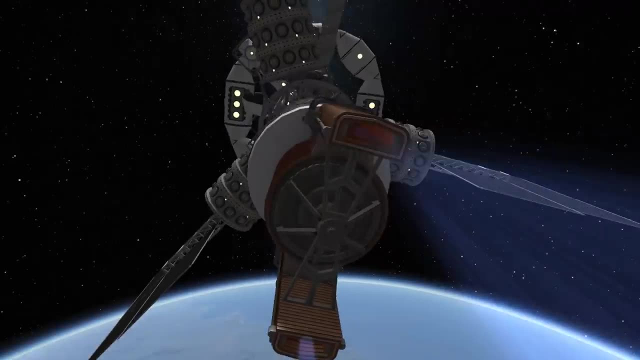 designs you get from a fission fragment rocket. You have a bunch of disks rotating quickly And as they move into this area, on the sides where you see the exhaust coming out of, that's where the reaction is happening, And when they move out, the reaction is being suspended and it's cooling off. 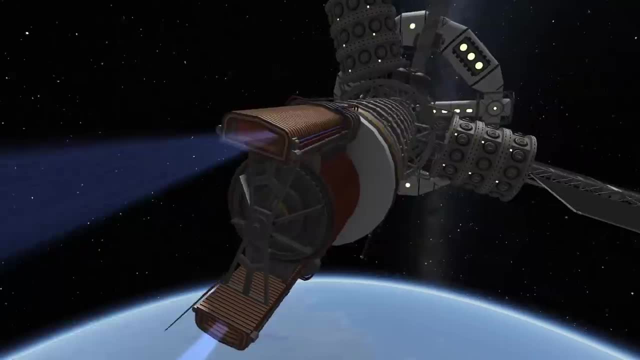 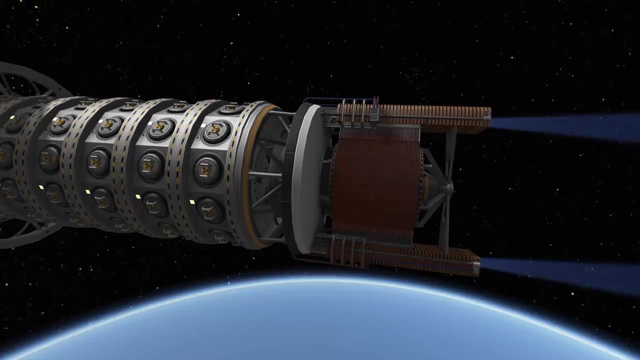 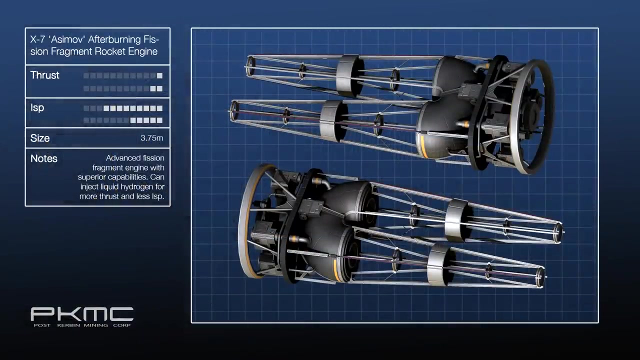 So it allows them to cool down without melting and also allows them to undergo fission in this region where the daughter products can be captured and converted into rocket exhaust. This is very, very high specific impulse engine, But it has really crappy thrust. So to get the good thrust you have, 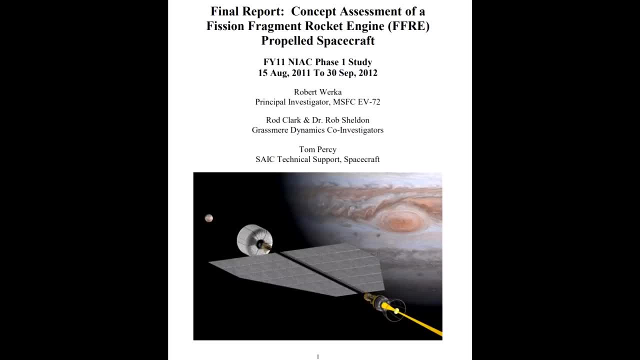 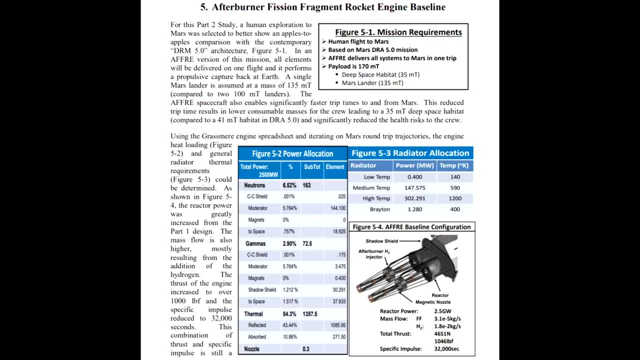 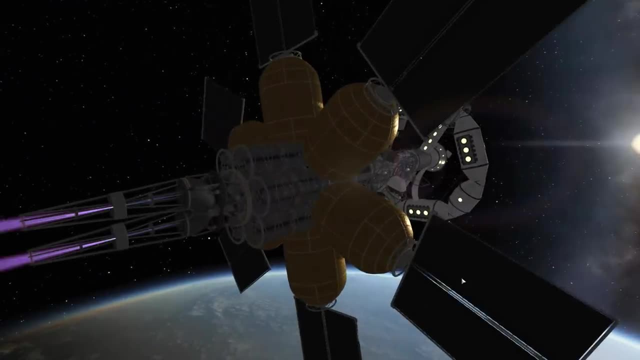 the afterburning fission fragment rocket engine, which again real NASA concept that has been studied and evaluated. The main idea again is that you have the fission fragment system but you have a mechanism by which you can dump hydrogen in there so that you can get extra thrust when you 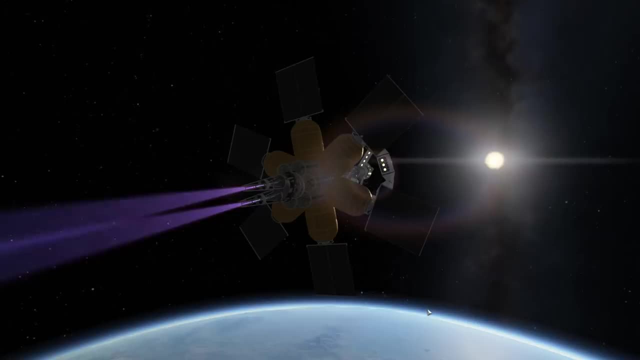 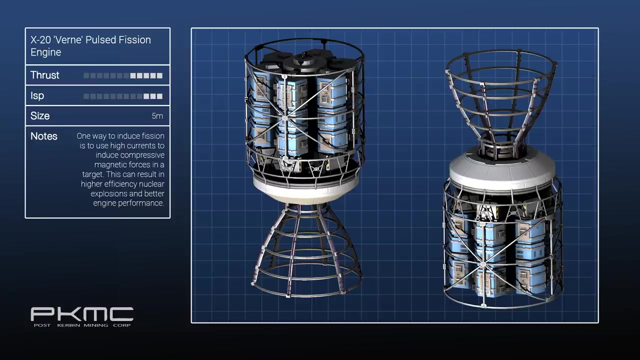 need a high thrust maneuver, And you can also get a high thrust when you need a high thrust maneuver. You can get ultra high efficiency when you only need to accelerate slowly. This is a pulsed fission engine And I wasn't sure what this was originally, but basically what you're doing is taking the core. 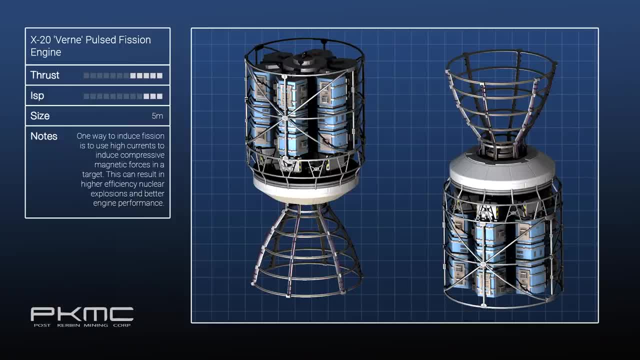 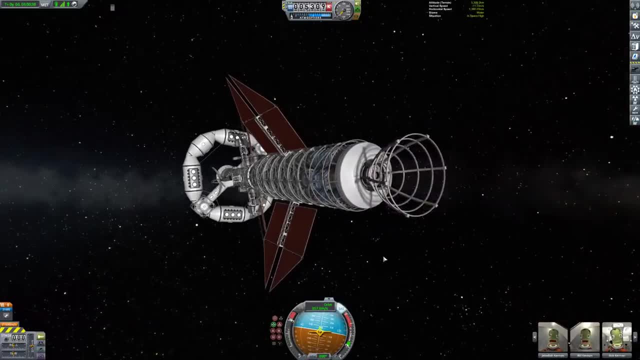 out of a nuclear weapon and making it smaller, And then, instead of having explosives to collapse it down and create the high depth density fissile material, you have a bunch of magnetic fields that collapse it down, So it's exactly like an Orion drive, except you don't need full on nuclear. 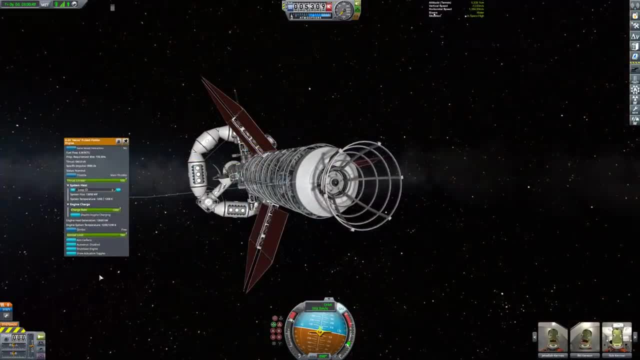 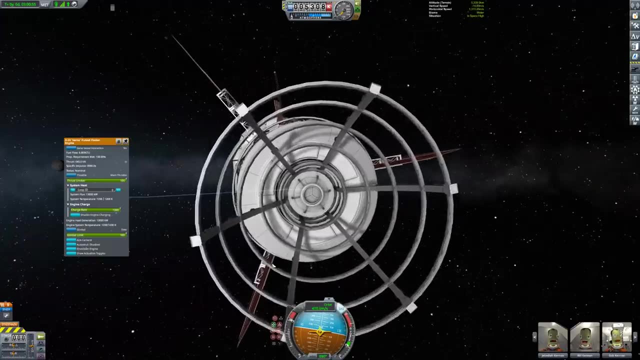 devices to generate the thrust, because most of the complex part of the device is in these magnetic fields. Now, according to what I've read, in theory they can use smaller critical masses because they can compress it more using these magnetic fields and they can hold the compression. 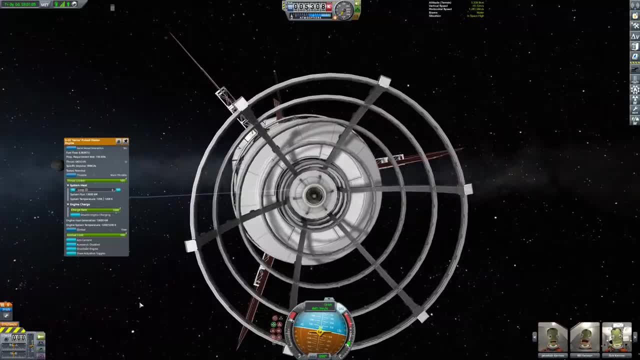 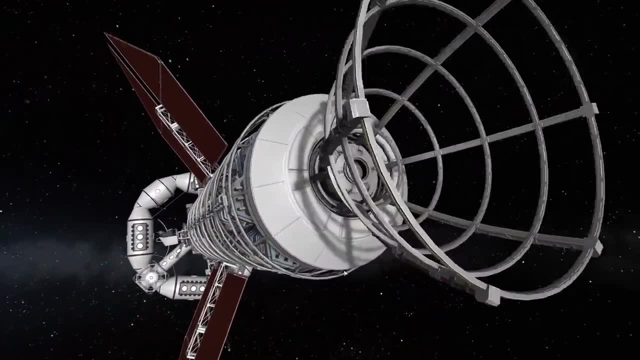 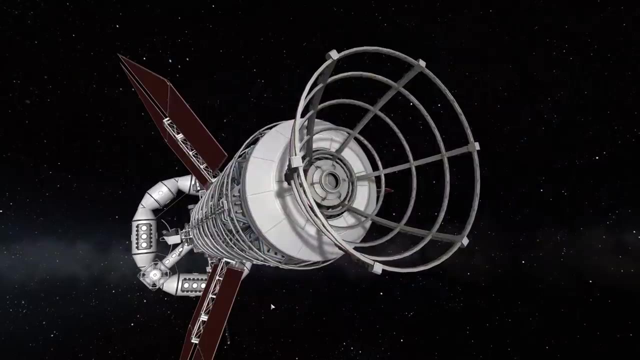 longer and get more efficiency. Also, some of the designs use some really interesting fissile materials. One used a curium 247, which is a long lived curium isotope. It has a half life, about one and a half million years, And it has a critical mass that's about 30% smaller than 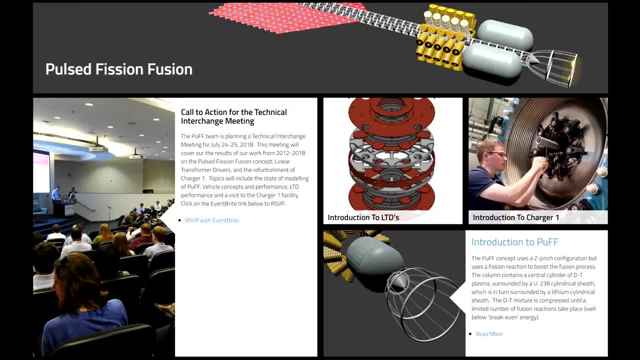 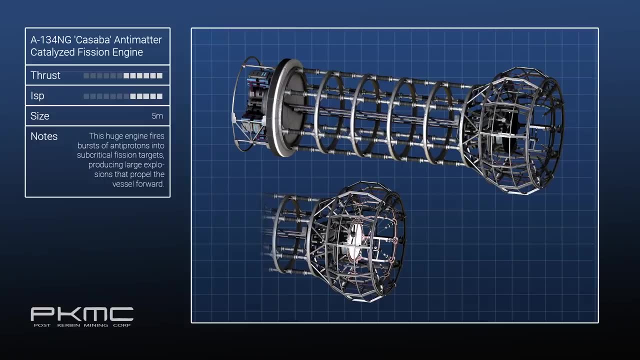 that of plutonium 239.. In a similar vein, you have the pulsed fission fusion engine, where you again use fission to start off your explosion, but you also have some fusion material in there to generate the majority of the energy Moving swiftly on. we have the antimatter catalyzed fission engine And 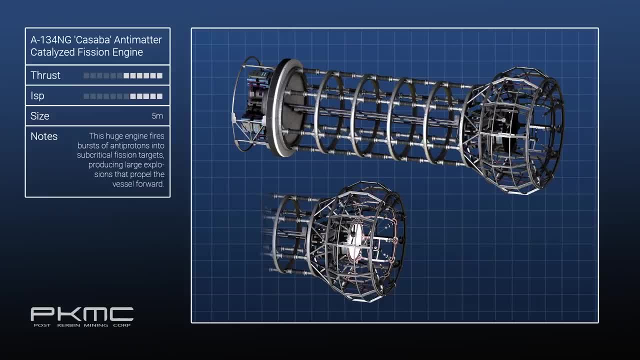 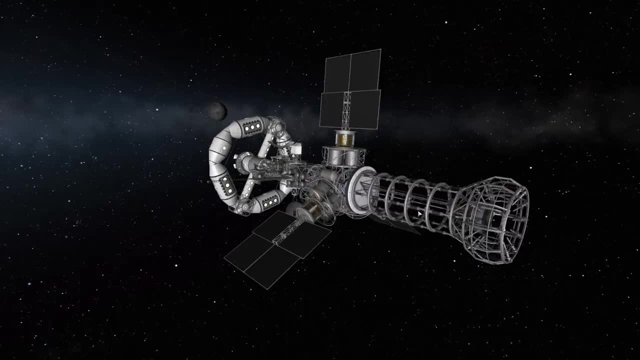 this is another pulsed engine where you're squeezing down a fissionable material target but you hit it with a fission. And this is a fissionable material target, but you hit it with some antiprotons And the antiprotons basically cause a whole bunch of fissions, and very quickly. 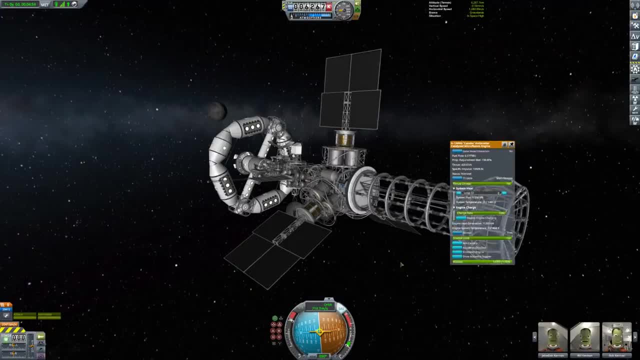 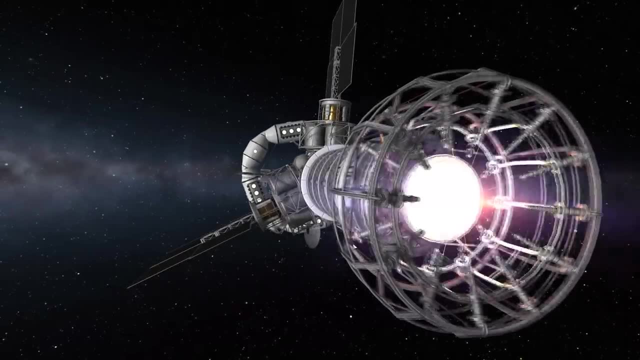 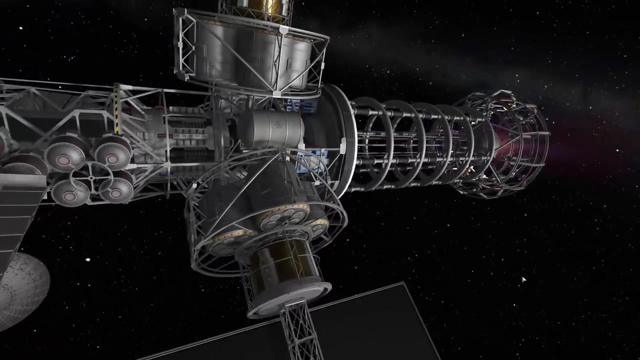 accelerate your reaction so you get a more powerful pulse out. And of course, this is us entering into the realm of the antimatter engines. Antimatter is fantastic because you get 100% conversion of matter into energy. The problem is getting large quantities off. it is very, very difficult. This 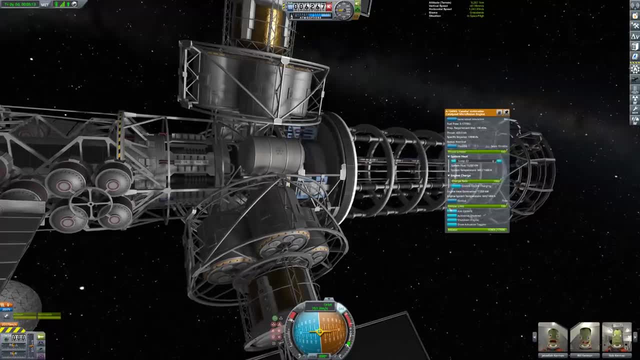 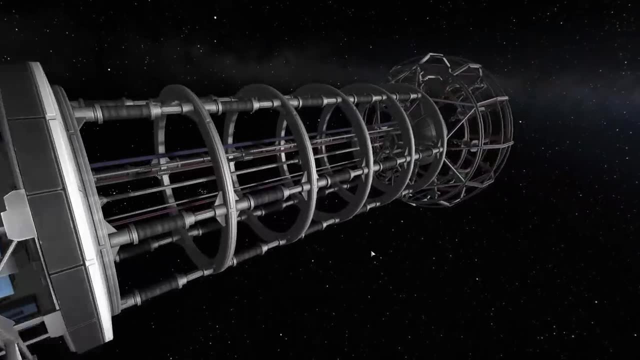 is why something like this, where you take a small quantity of antimatter and you put it in a fission or a fusion process and you use it to release more energy from, say, a fission or a fusion process. So the antimatter is there just to give you a little extra kick, a little extra performance. 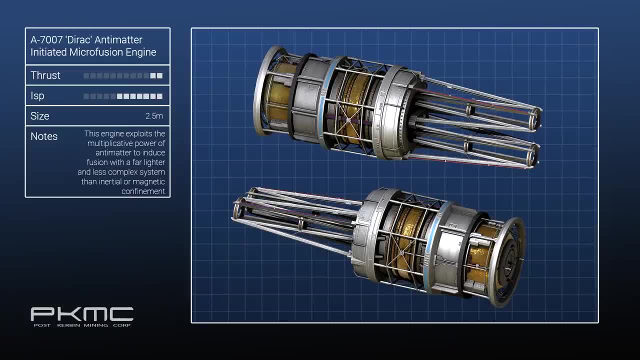 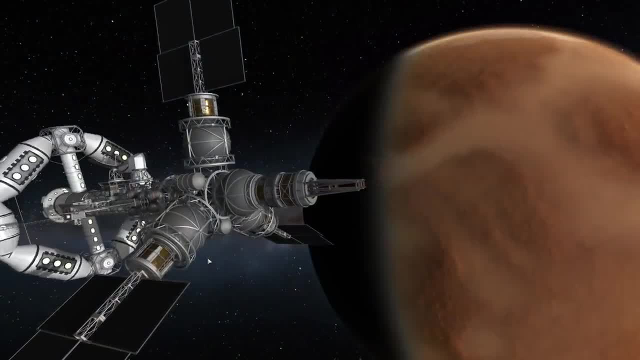 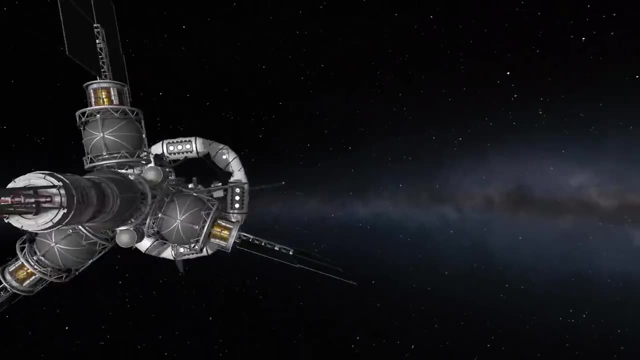 from your other energy sources. And in the same vein we have the antimatter-initiated microfusion engine And in this concept you have a droplet of liquid deuterium, you surround it by uranium or some other fissile material and then hit it with a bunch of antimatter And that causes. 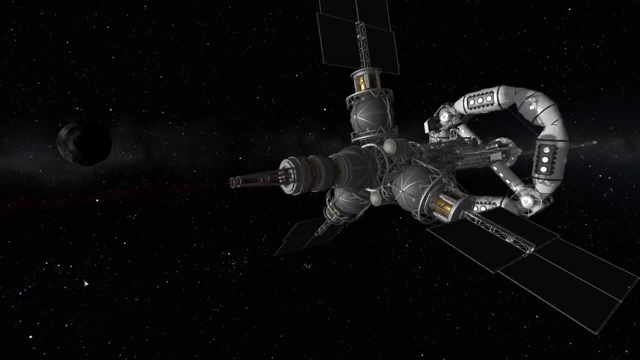 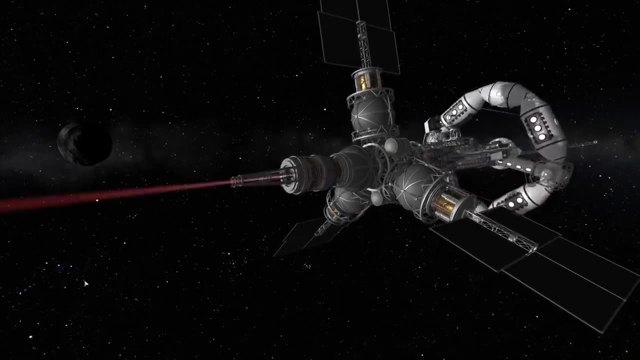 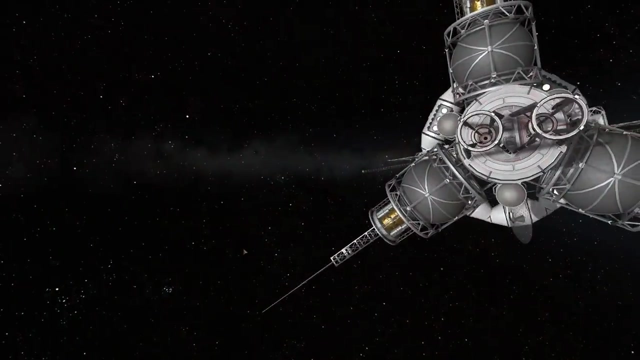 fission in the uranium, which causes the compression of the deuterium and fusion, You get a little explosion coming out of it. So while you're using antimatter and fissile materials to start off the reaction, most of the energy does come from the fusion. And finally, if you somehow 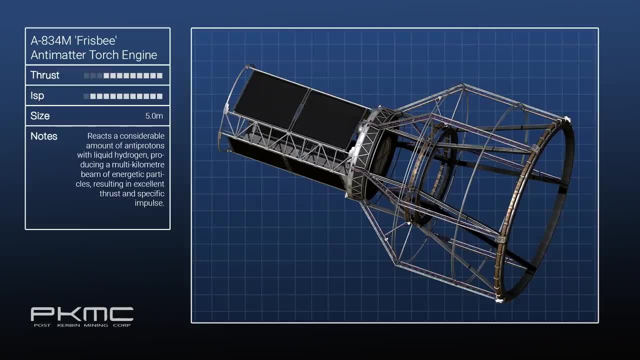 were able to get around that problem of conservation of baryon number and manufacture large quantities of antimatter or counter-matter, you could use the antimatter-initiated microfusion engine to capture it from somewhere. Then you could have a pure antimatter drive. This is the 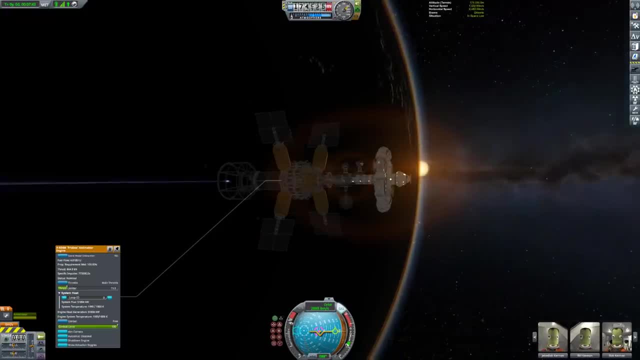 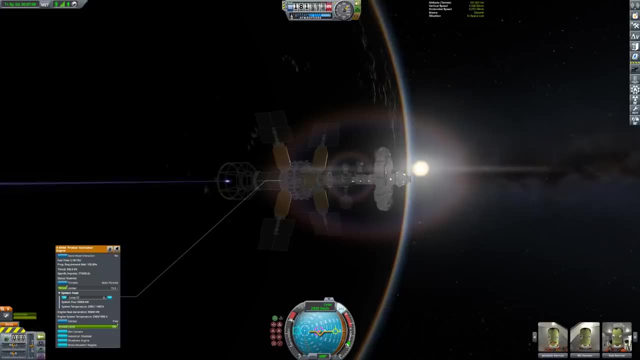 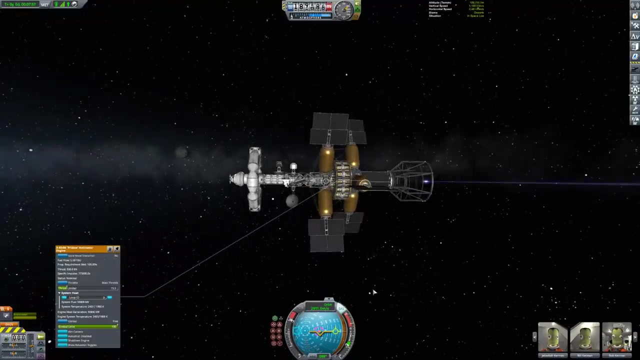 Frisbee antimatter torch. I don't know why it's called Frisbee, but yeah, this actually comes in various sizes. within the mod There's the little dinky short one, and the main difference appears to be the longer they are, the more cooling they have. So this one I actually didn't realize when. 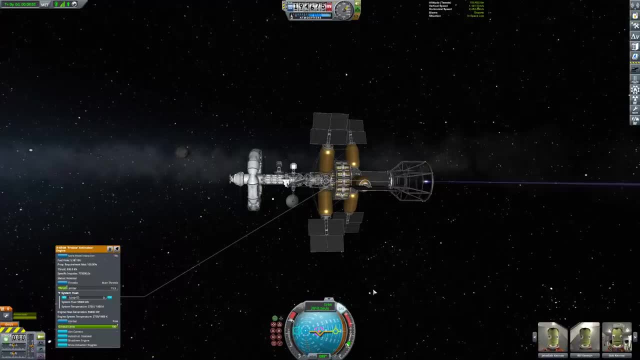 I launched it, I didn't have enough radiator panels to be able to keep the thing cool. One of the things that's important in a lot of future technologies for spacecraft propulsion is that they generate a lot of energy and they need a lot of radiators to be able to keep the spacecraft cool, keep the system cool.